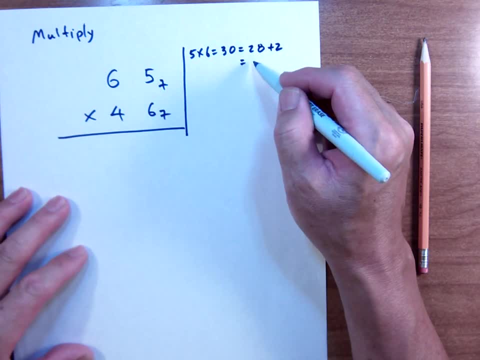 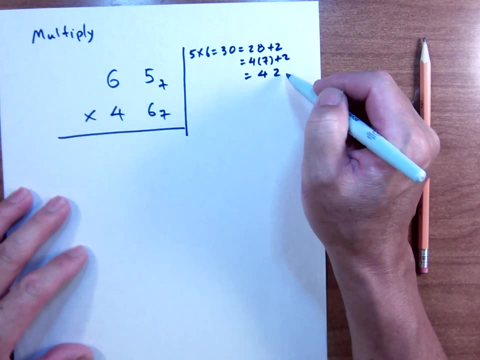 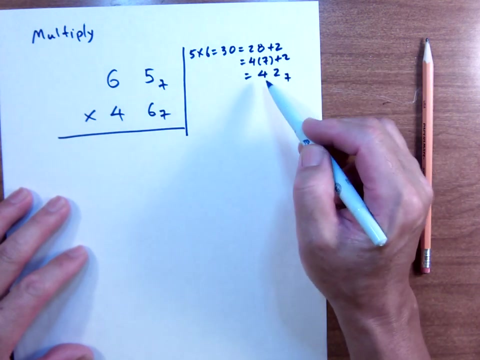 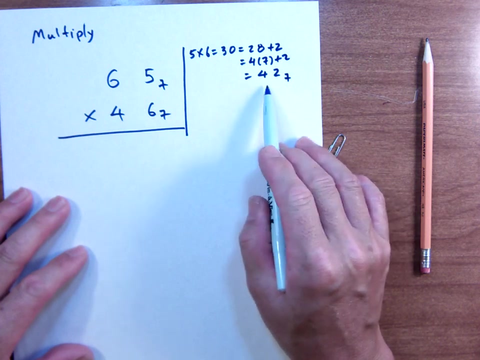 Plus 2 is equal to 30. Therefore, since 28 is 4 times 7, 30 is written as 4 to base 7.. Okay, I hope you can follow that I'm not going to really go through all the details for every single multiplication, So please, if that was a little too fast, we'll go back and make sure you understand this process. Alright, so we're going to write the 2.. 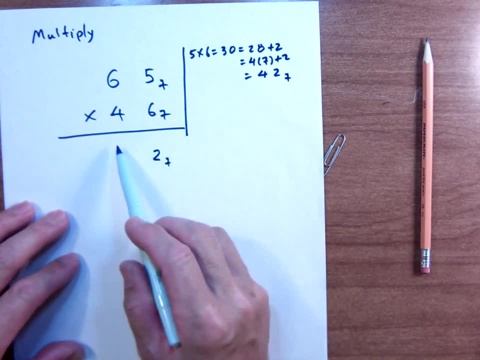 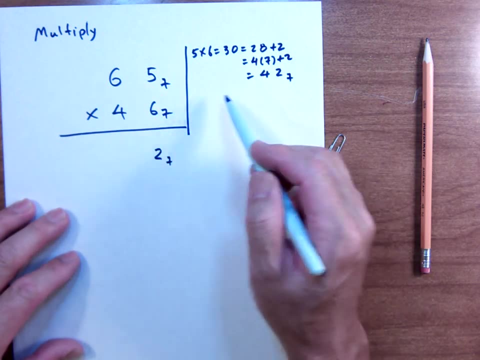 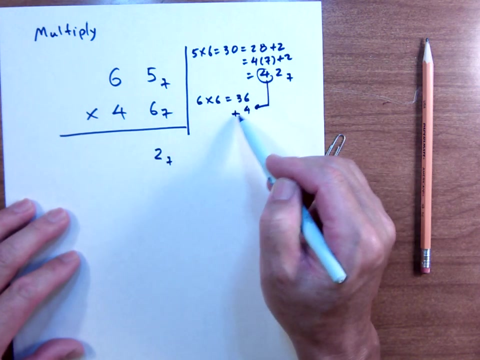 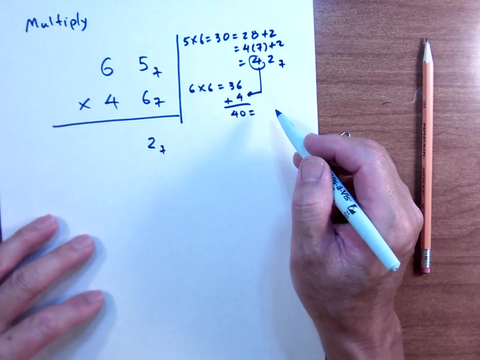 Okay, and again, leave a little space here, Because when we add, you don't know, Maybe we will need to carry over. Okay, next one is 6 times 6.. So we'll do 6 times 6. That's 36.. Remember this: 4 now does need to be carried over, Which gives us a value of 40. And now 40. Again needs to be converted to base 7.. And the closest multiple of 7 to 40 is 40. 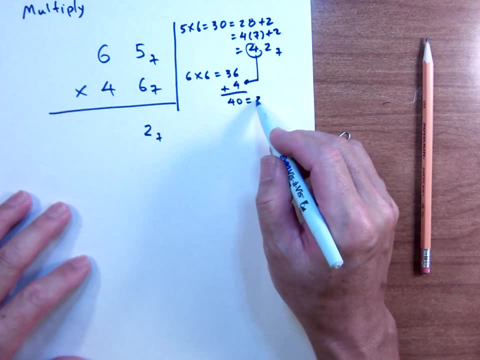 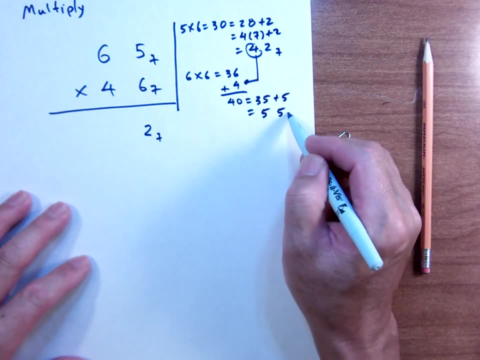 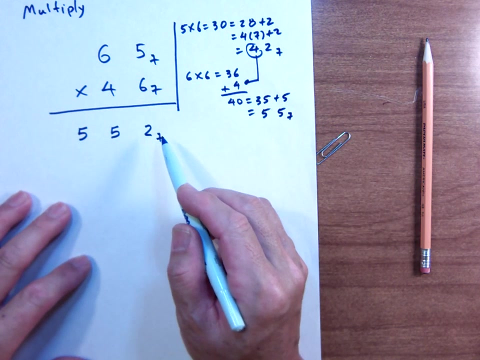 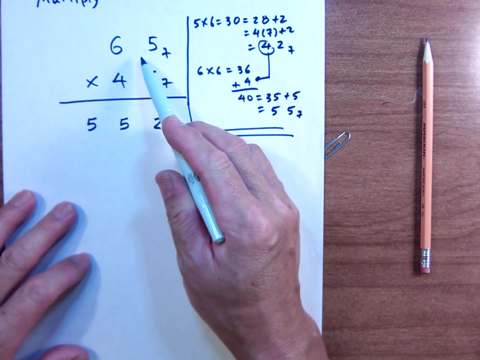 35.. So that was going to be. I'm going to write that as 35 plus 5.. And since 35 is 5 times 7, this will be 5, 5 base 7.. Okay, Alright, so that is the result of the first row, And let's go. Okay, And our next number we're going to multiply is now by 4.. So 5 times 4 is 20.. 20 is. 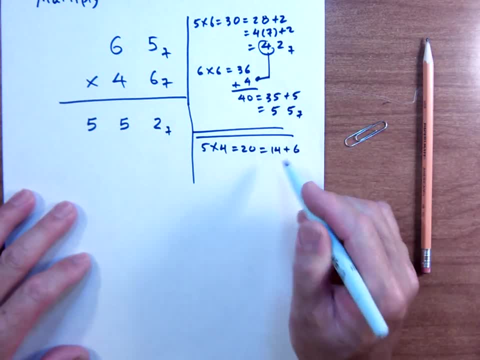 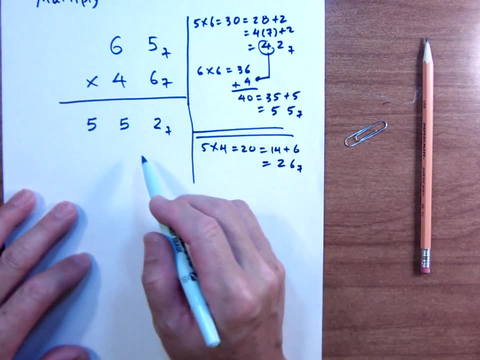 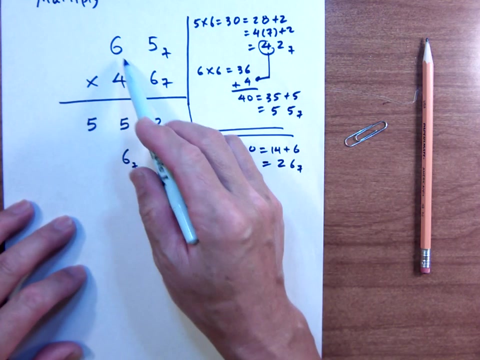 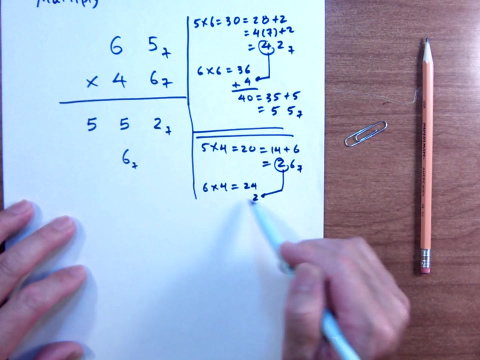 14 plus 6.. Okay, Again 14, because that is the multiple closest multiple of 7.. So that will be 2: 6 base, 7.. So write the 6.. Don't forget to stagger one column over. Okay, And our last one is 6 times 4.. 6 times 4 is 24.. Carry over this: 2. Gives us 26. And 26. 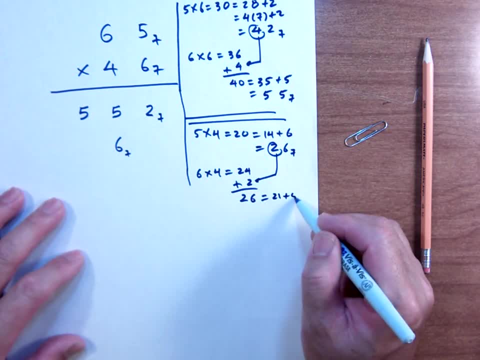 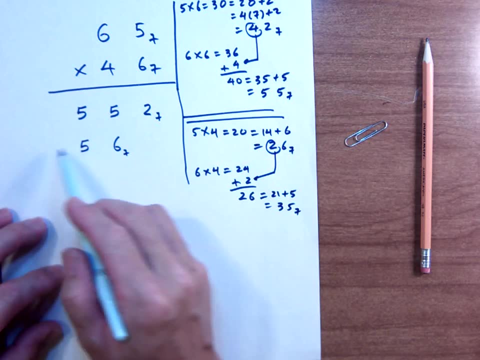 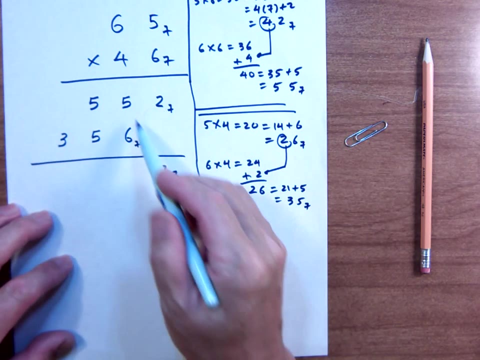 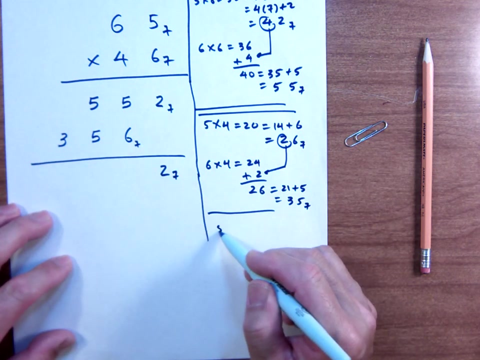 is going to be 21 plus 5.. So that will be 3: 5 base 7.. Okay, So write the 5.. Write the 3.. Now we need to add this 2 rows down. Okay, So 2 will come straight down: 5 plus 6.. Hope you didn't forget to add the addition in base 7.. 5 plus 6 is 11.. 11 is going to be written as 1- 4.. 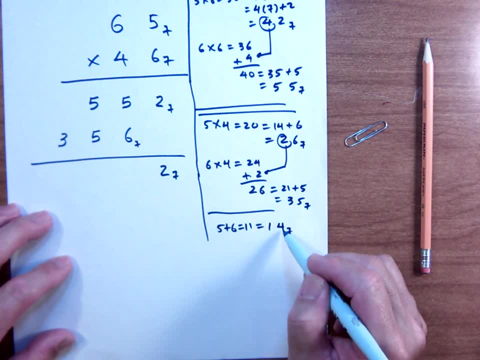 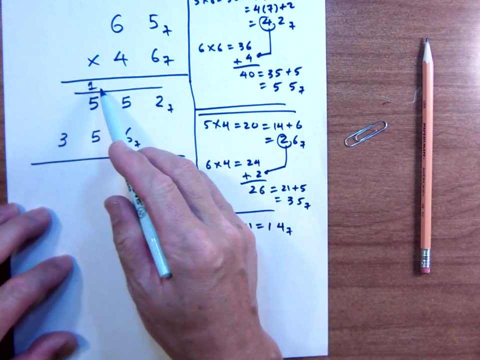 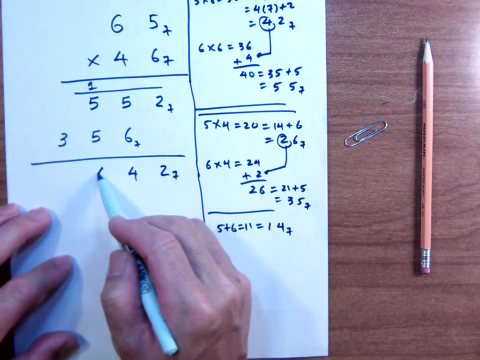 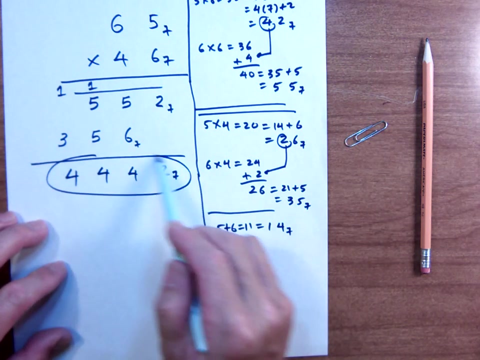 4 base 7.. Since 11 is 7 plus 4.. So we write the 4. Carry over the 1.. Next column: 1 plus 5 plus 5 is 11.. Again, 11 is going to be 1, 4.. We already did that. So 4 carry over 1. And 1 plus 3 is 4.. So there you have it. That's our answer. 4, 4, 4, 2 base 7 is the product of multiplying the. 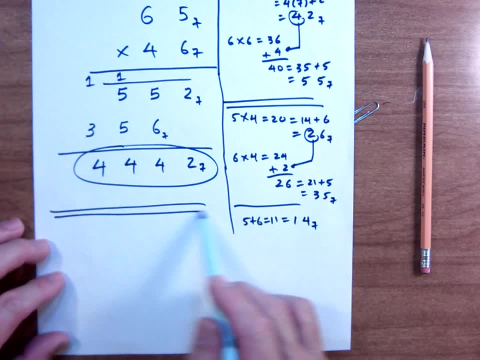 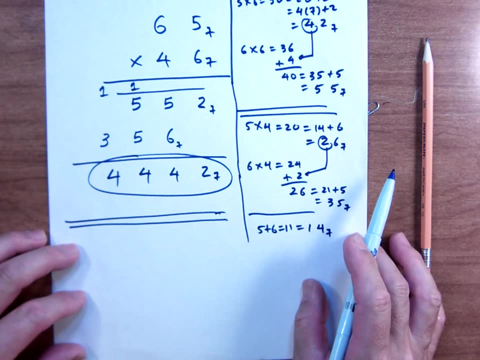 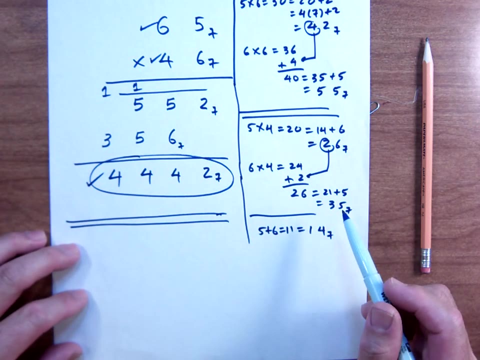 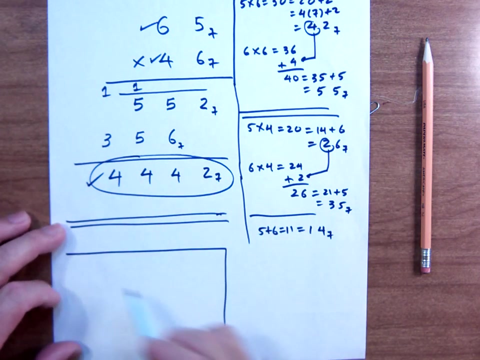 2. Okay, Now I'm going to quickly show you how we can check your answer. All right, And the only way for us to check this is by converting all 3 numerals to base 10.. What 3?? 1 here, 1 here And the solution. Okay. So here our numbers go up to 4 places, So we do need to create a chart that we've seen before: 4 base 7.. 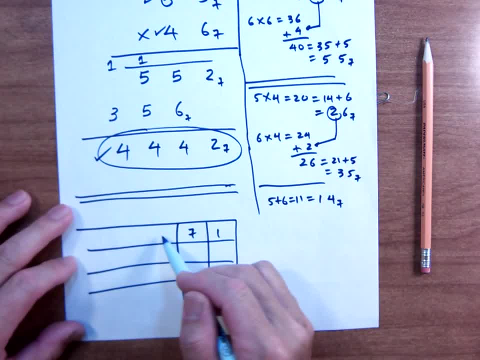 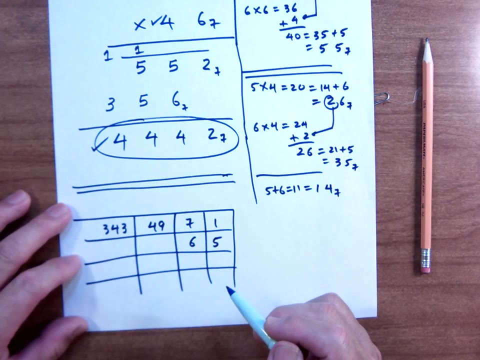 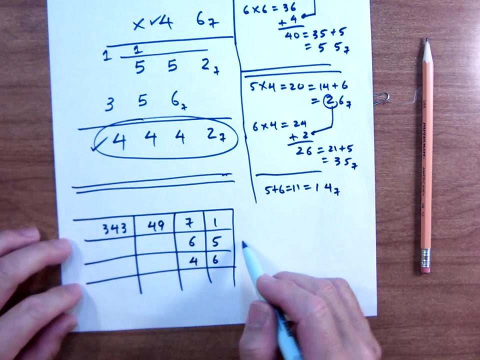 1, 7.. 7 square is 49.. 49 times 7 is 343.. Again, those are so-called the position base values for base 7.. Okay, Let's enter our number in question: 6, 5 was the first one, 4, 6 is the second. Again, what we're going to do is we're going to convert these 2 base 10 numerals. 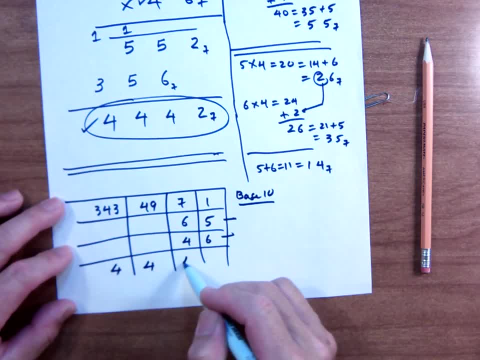 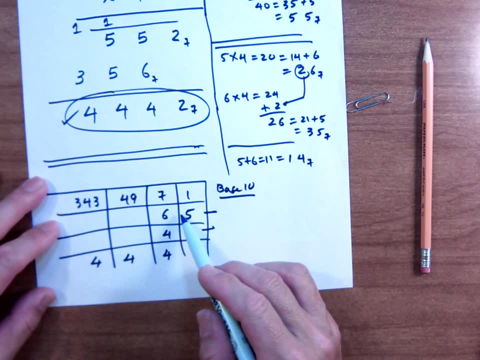 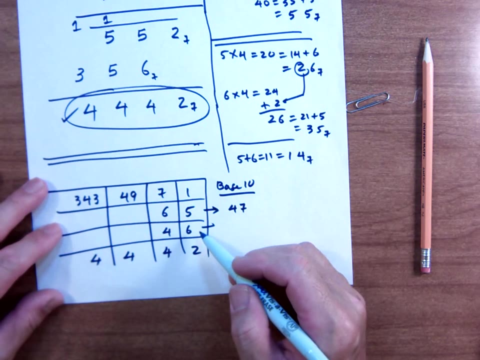 And our answer was 4, 4, 4, 2.. All right, Okay, So let's take our calculator. Well, actually we don't really need a calculator for all these. 7 times 6 is 42.. 42 plus 5 is 47. Okay. Second one: 7 times 4 is 28.. 28 plus 6 is equal to 34.. Okay, So eventually we will multiply 47 times. 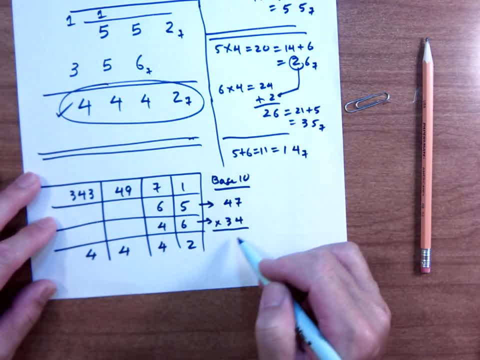 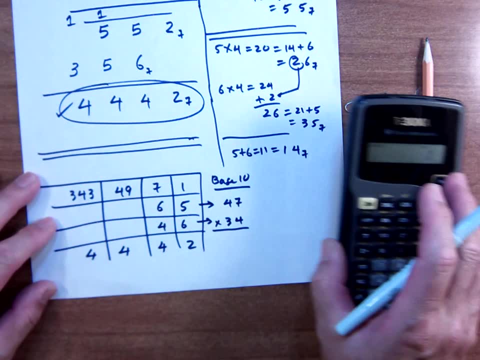 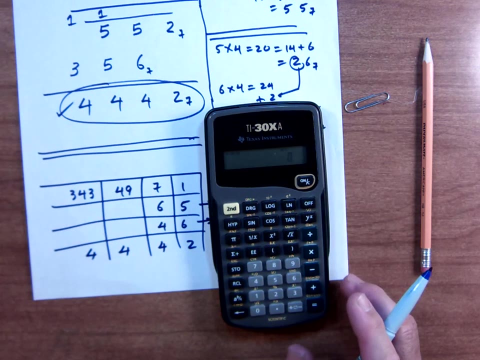 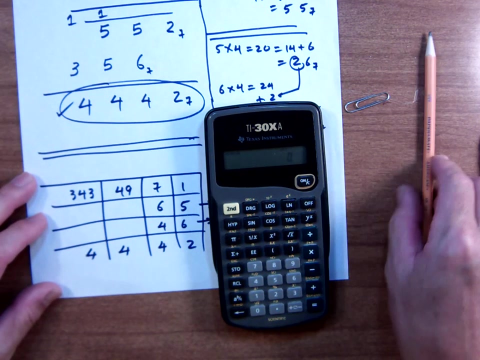 34 in base 10.. And hopefully that product equals the conversion that we will be doing for this last numeral, That one. I will use a calculator. So 4 4, 4, 2.. Okay, Let's see. I hope you can see the screen. Let me zoom in a little bit Zoom. Can I zoom in while you are in recording mode? All right, So I hope you can see this: 343 times, 4.. So I'm going to go. 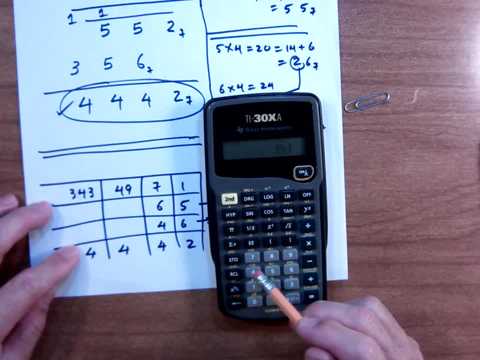 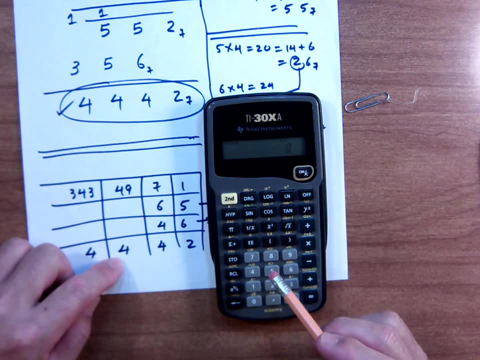 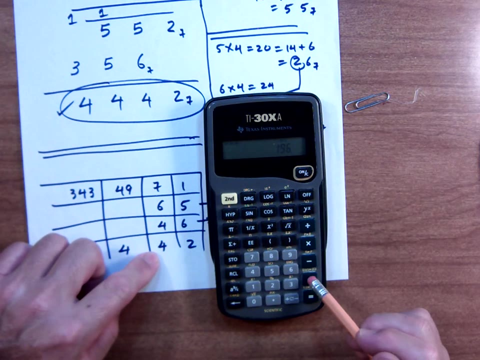 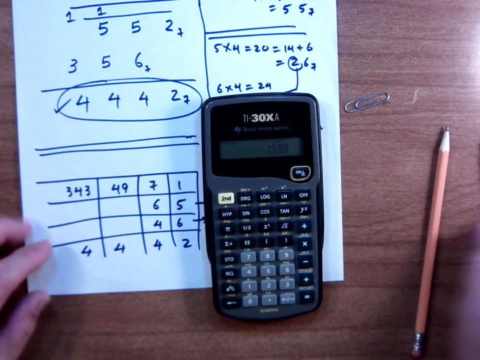 343 times 4 plus Next is 49 times 4.. I'm going to open up parentheses. Open parentheses: 49 times 4.. Close parentheses: Plus That's 28 and 2, which is 30. 30 equals 1598. So it's a little bit small. Okay, You can see. 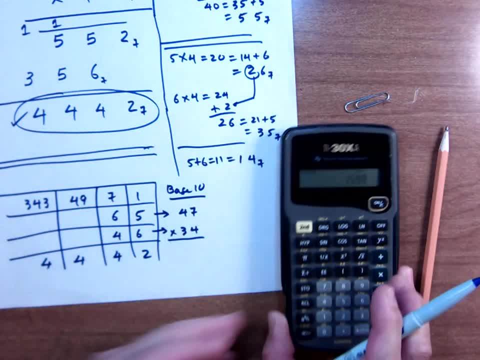 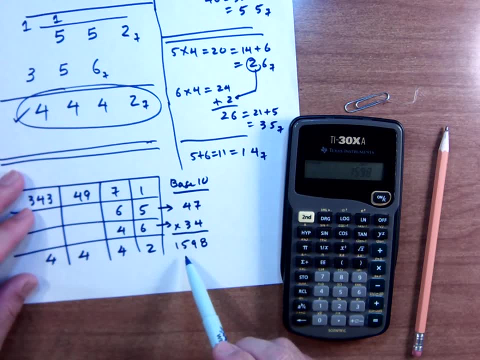 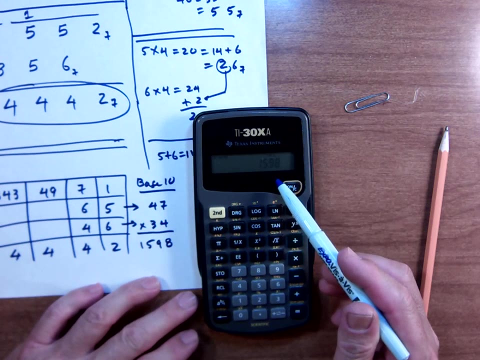 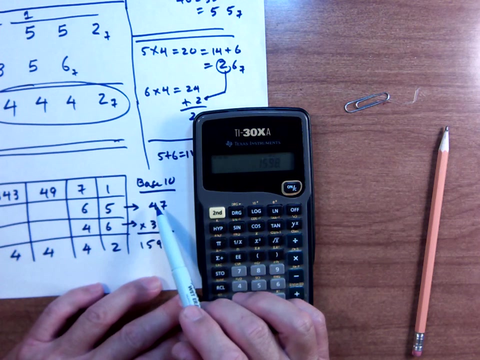 that 1598. Okay. Okay, Is it true that 47 times 34 is equal to 1598?? Well, instead of multiplying, what you can do is- since I already have 1598 on the screen, I'm just going to divide this by either of the two, And the result should be the other one. So, if I divide this by 34, I should get 47.. So let's do that. Divide this by 34 equals 47 times 4.. 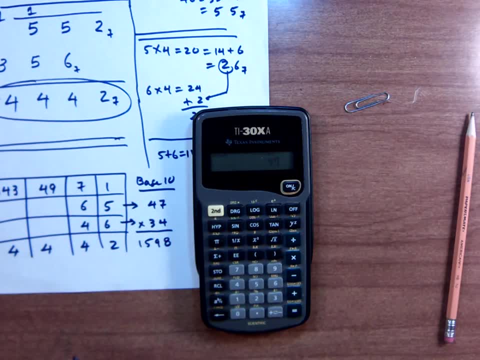 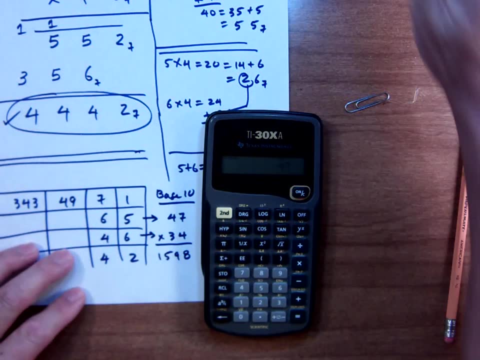 And there you have it. So this verifies that our answer of 4, 4, 4, 2 base 7 is indeed the correct result. All right, That's it.